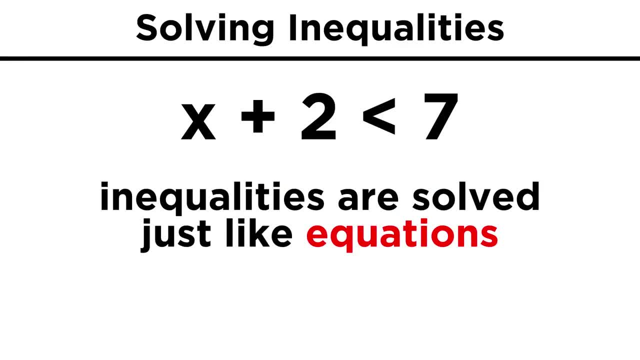 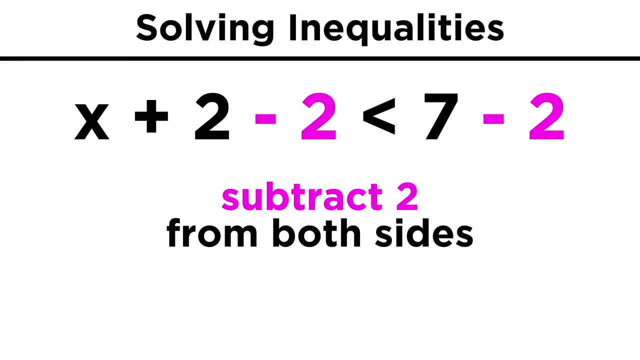 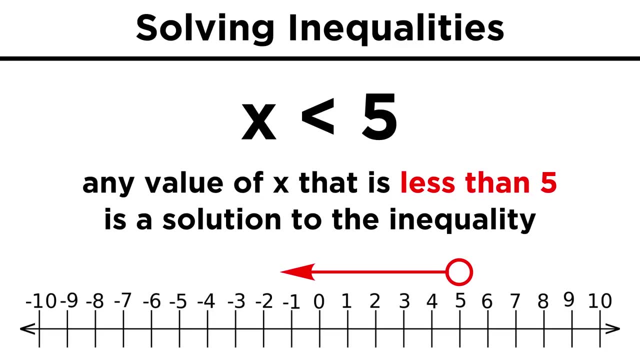 We will see inequalities set up, like some of the equations we've seen as well. How about X plus two is less than seven. As you might expect, all we do is subtract two from both sides, which gives us X is less than five. so any value less than five is a solution, while five or above is not. 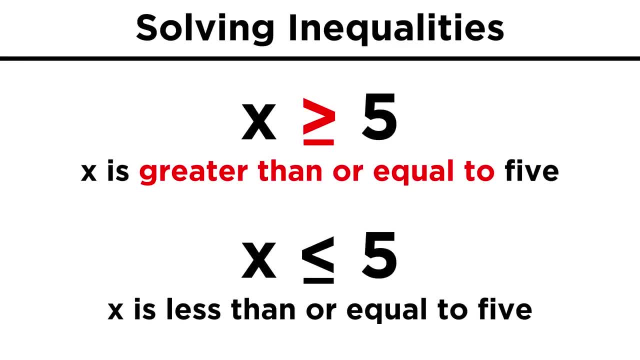 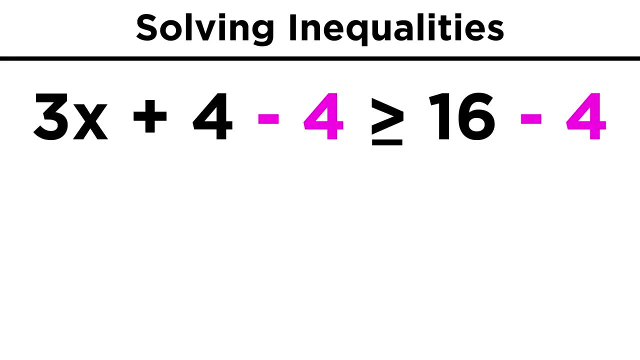 We will also see these symbols which mean greater than or equal to, And less than or equal to. These work the same way as the other symbols, except that they include the specific value shown rather than excluding it. If we have three X plus four is greater than or equal to sixteen. we subtract four from. 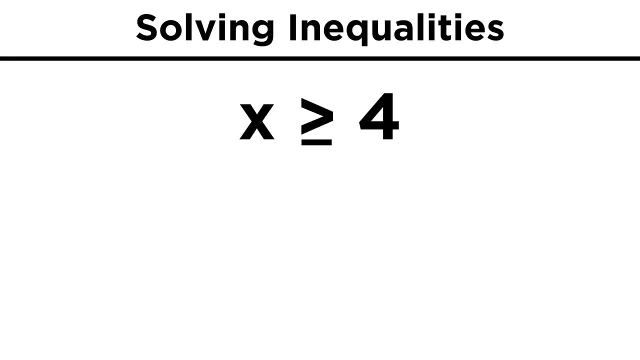 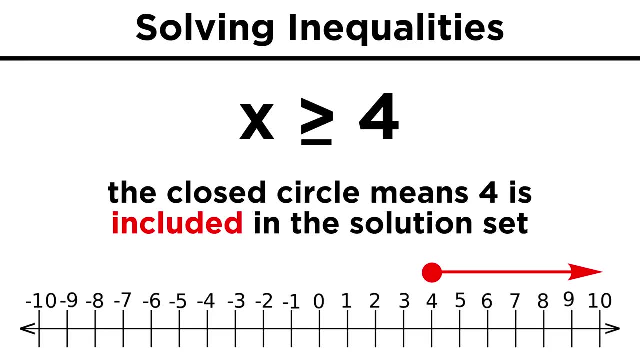 both sides, then divide by three and we get X is greater than or equal to four. Now, on the number line, we represent this with a closed circle, meaning that it is filled in rather than empty, to represent that the number four is included. 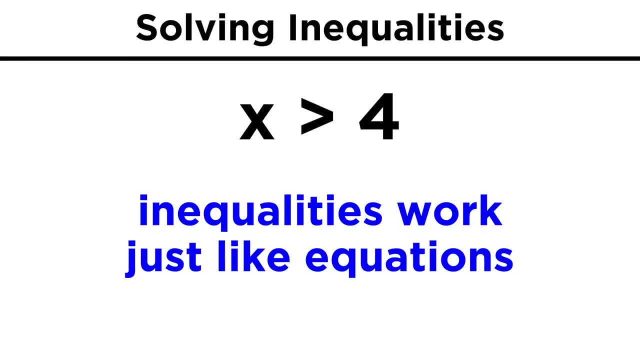 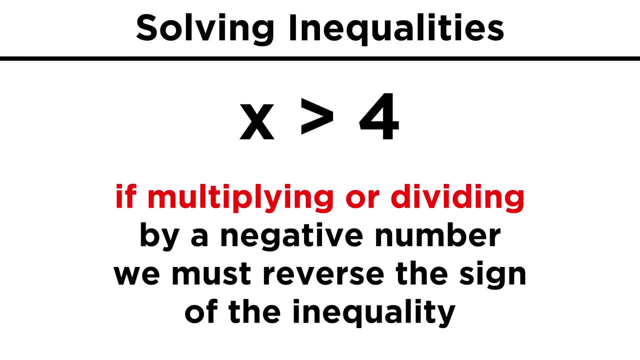 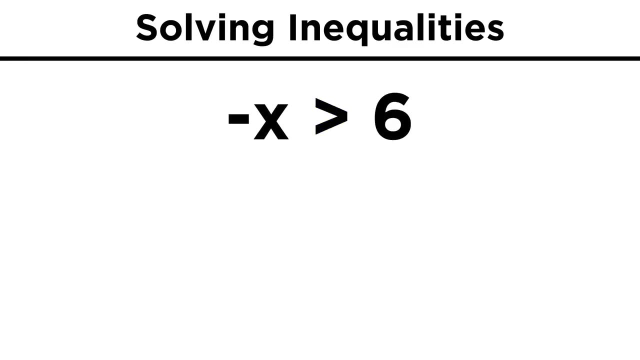 So everything here works the same way it does with equations, but there is one difference we need to point out. If we are multiplying or dividing by a negative number, we need to reverse the direction of the inequality symbol. For example, if negative X is greater than six, we would either multiply or divide both. 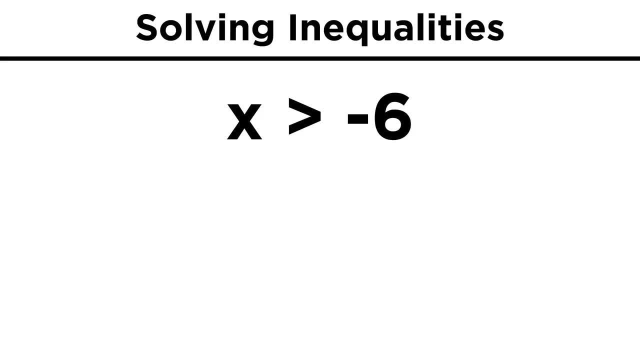 sides, by negative one to get X. but if we do that, we have to switch the greater than to a less than X is less than negative six. To see why this is the case, let's test this solution. Take the first version and plug in negative ten. 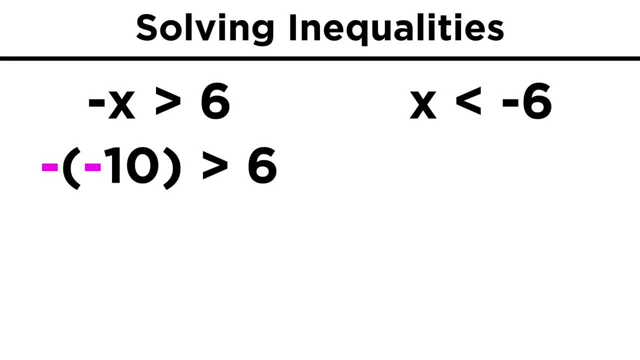 The negative version of negative ten, or the opposite of negative ten, is ten, and that is indeed greater than six. Now, with our revised version, negative ten is also less than negative six, so we can see that this flipped version is indeed the correct counterpart. 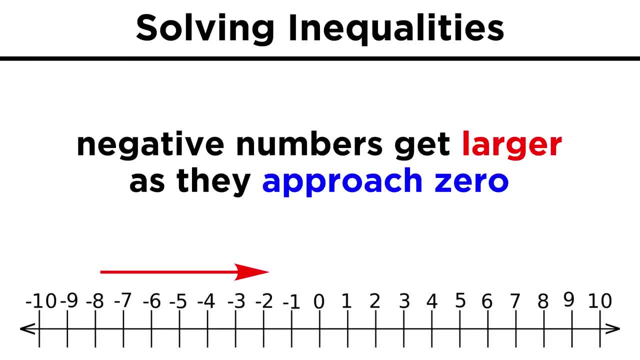 One way of rationalizing this is by looking at the equation First. let's remember that negative numbers closer to zero are larger than negative numbers farther away from zero. so although it may for a moment seem like negative ten is bigger than negative five, it's actually the other way around.